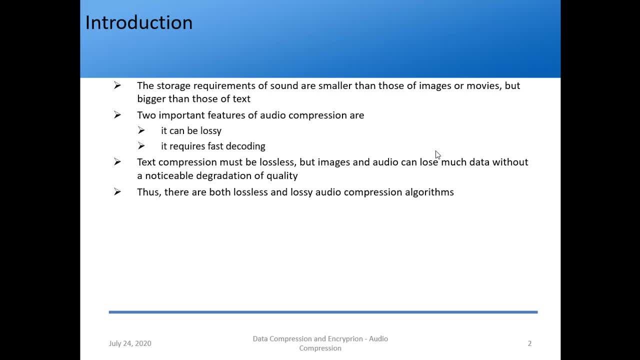 So if the player says decoding 1%, 2%, 3%, 4%, etc. So that won't work out right, Because we want the file to play as soon as we click on the file. right, So fast recording is very important. 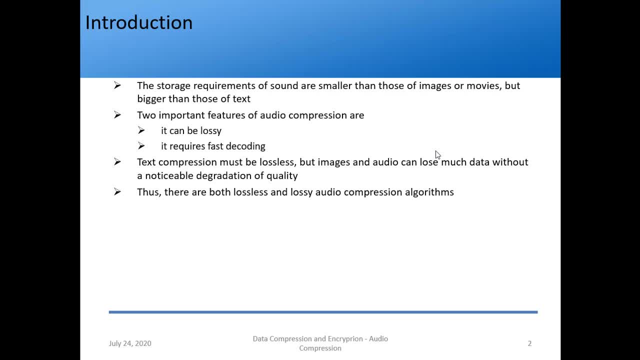 But what about the encoder? Encoder can be 100 times more complex than the decoder, Because it is done beforehand, right? So if you have a file, means it's already encoded file. That is what we mean here by complex right. 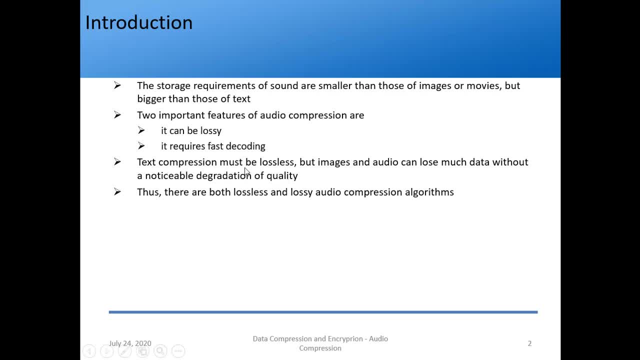 So text compression must obviously be lossless, Because if there is even a small alphabet change it might create problems, right? But images and audio can lose much data. Thus there are both lossless and lossy audio compression algorithms, right. 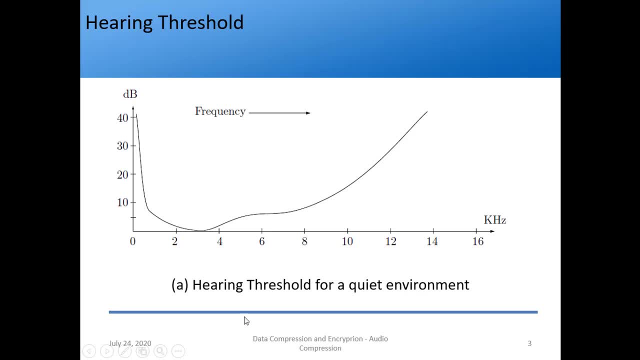 So then this is a very important slide. So what does this give? This gives hearing threshold And remember, it is for a quiet environment. I forgot to mention this in the last lecture. So x axis is frequency, Y axis is the hearing threshold in dB. 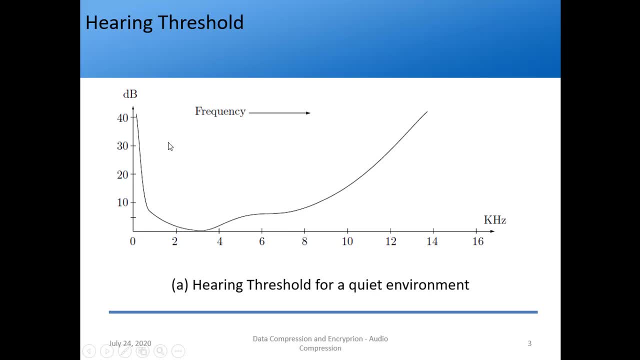 So this is the demarcating line. So whatever is above the line, those levels can be heard by the ear right, And whatever is below cannot be heard right. So this can be compressed Because this, anyways, we are not going to hear. 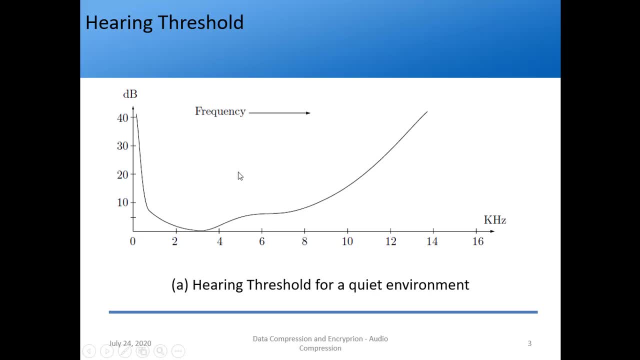 So no need of them keeping in the file. So this is what we thought about hearing threshold right, And we also said from 2 kHz to 4 kHz. the ear is very sensitive Because it can hear levels up to the levels of 0 dB also almost. 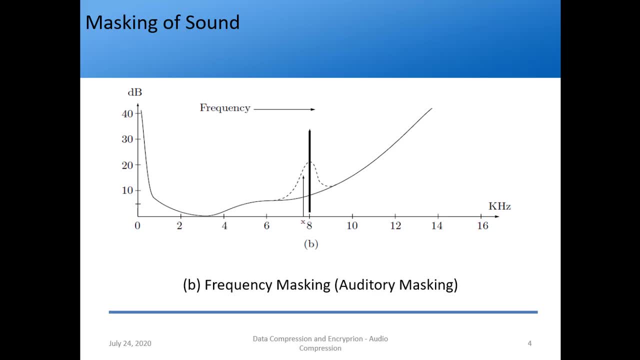 So then we studied masking of sound, Again very important from exam point of view. So there were two types of masking: Frequency or auditory masking, And the second was temporal masking. So what was frequency masking? This is our usual last slide diagram only. 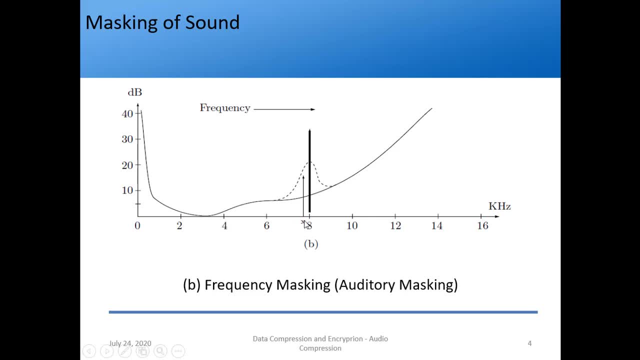 Hearing threshold So at 8 kHz. if we have a very high sound, For example that of a cannon Or a supersonic jet, as we took the example yesterday, What it does? It increases the hearing threshold in the vicinity. 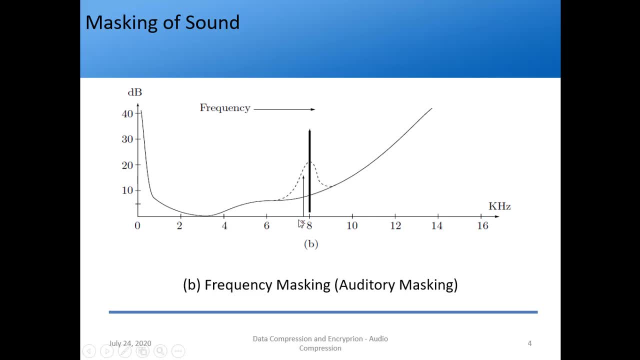 So if in the same increased threshold in the vicinity, If we have another sound at a frequency x, What we see It is below the threshold right. So ideally it should have been listened by us. But since there is a huge other sound, 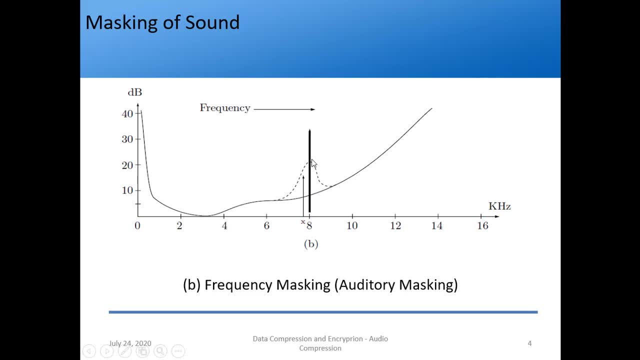 It is getting masked by this higher black thin line, right? So this is what is frequency masking. So an efficient encoder should do what It should not: encode this frequency x. That is this sound, right? So this is how compression can be achieved. 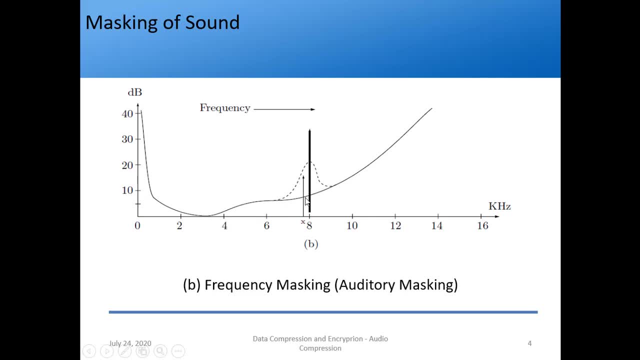 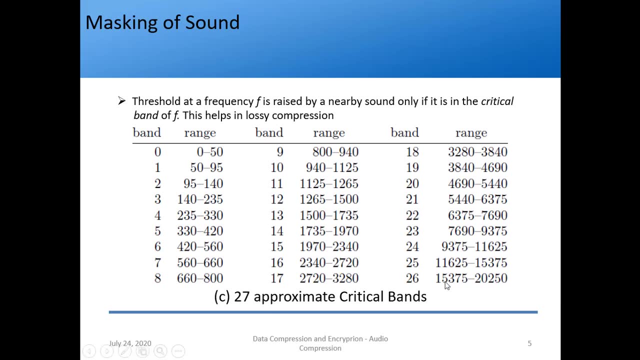 Because, anyways, we are not going to hear, So no need to keep it right. So this is what? frequency or auditory masking. So next we talked about frequency, or 27 approximate critical bands. It is not that important from exam point of view. 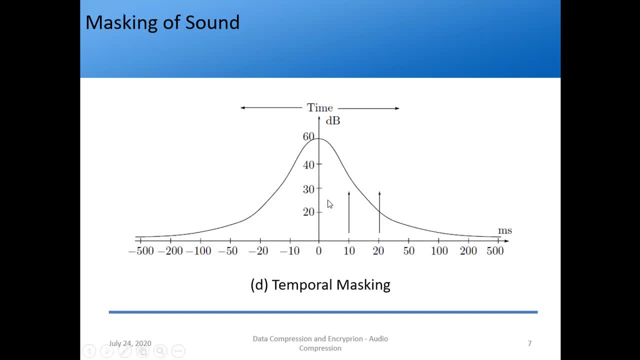 So we will skip this. So then, we studied temporal masking. So if you have a very high sound, What is meant by temporal? Temporal means depending on time. That is why our next exercise- now we have time. Previously we had what? 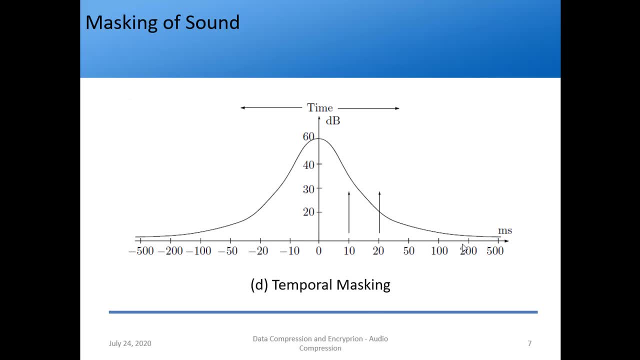 Frequency. So it was frequency masking, right? So if I have a sound, very high, sound at t equal to 0 milliseconds, That if it has a effect further down till 500 milliseconds also. That is what this graph shows. 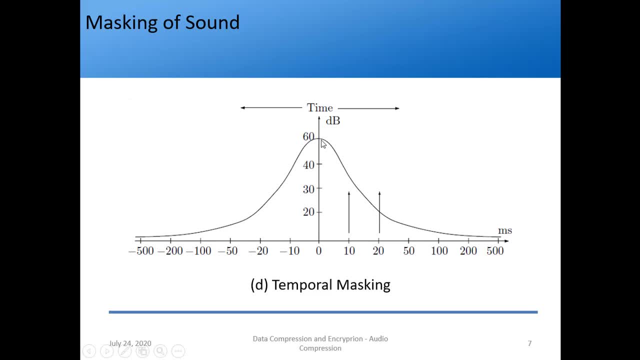 So if we have another sound at 10 milliseconds, It is getting clearly masked away by this high sound. But the sound at 20 milliseconds is not getting masked right. It is clearly seen here. So these lines indicate this. So these lines indicate the sounds. 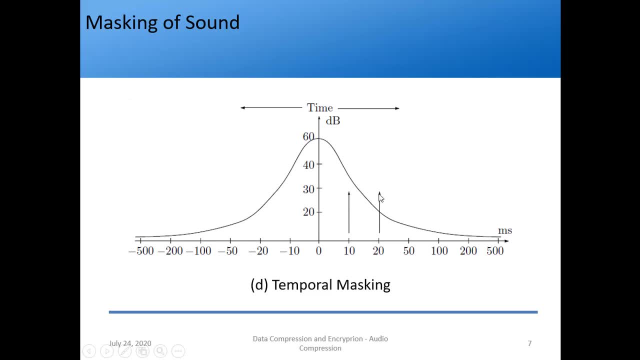 So 10 milliseconds is getting masked and 20 milliseconds is not getting masked. So again, our encoder should be able to see this. So it should mask the 10 millisecond sound but not mask the 20 milliseconds sound. So this type of masking is based on time. 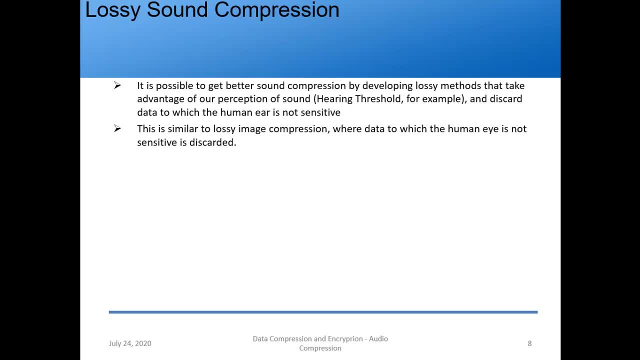 So it is called as temporal masking right. Then we started with lossy sound compression. So it is possible to get better sound compression by what? Developing lossy methods, So lossy methods that take advantage of our perception of sound. 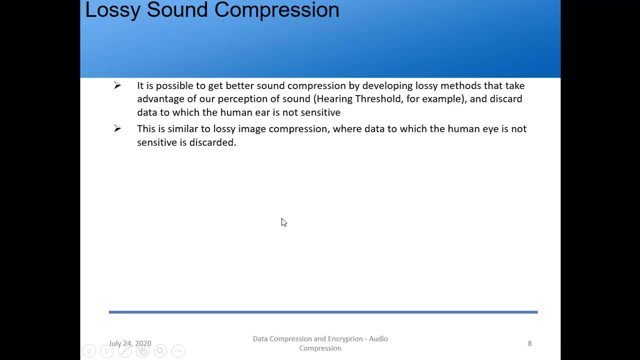 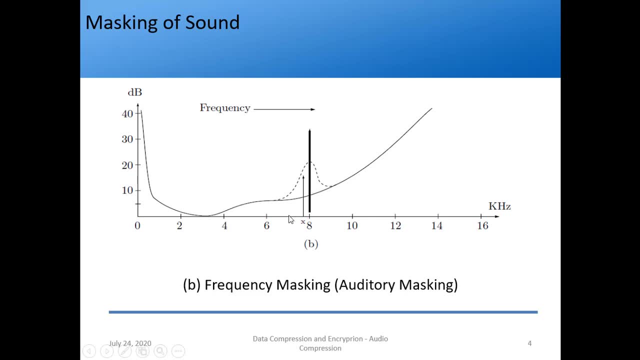 So hearing threshold graph we saw. So whatever is below that should be removed from the file. And if you take the example of frequency, masking, this frequency at x kilohertz should be removed Because they are not going to be heard. 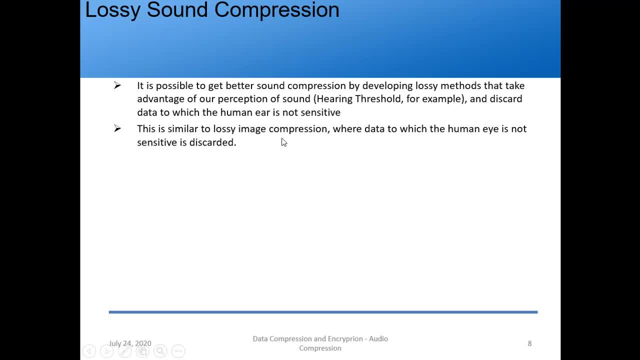 So this is perception of sound, right? So this is similar to lossy image compression. So then we studied silence compression. What is it? So we treat the small samples as if they were silenced. If there is silence, nothing needs to be transmitted, right? 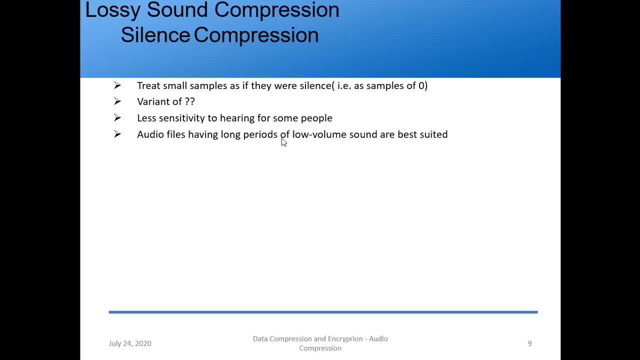 So this is silence, compression, So, and it is a variant of RLE, So we saw further some things regarding to that. So then we took the very important topic of compending. So what is compending? It is nothing but compression and expansion. it stands for 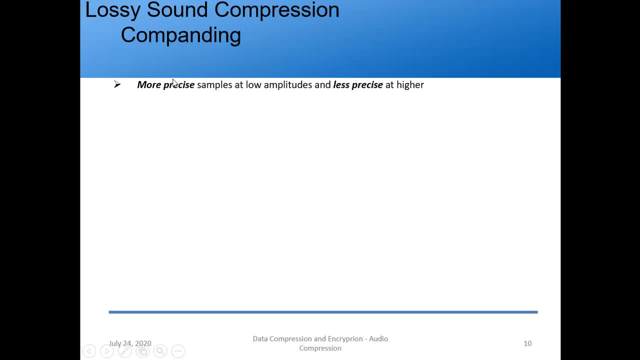 It is taken from those two words. So we said that at low amplitudes very high information is contained. So there should be more precise samples at low amplitudes and less precise at higher amplitudes. So what should be the quantization here? 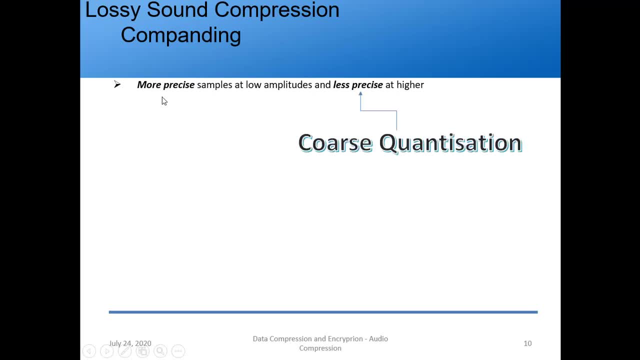 It should be finely quantized, right, And less precise should be coarsely quantized. So then, this is not important. So then, compending is non-linear. Why is it non-linear? Because more precise samples are at low amplitudes and less precise at higher amplitudes. 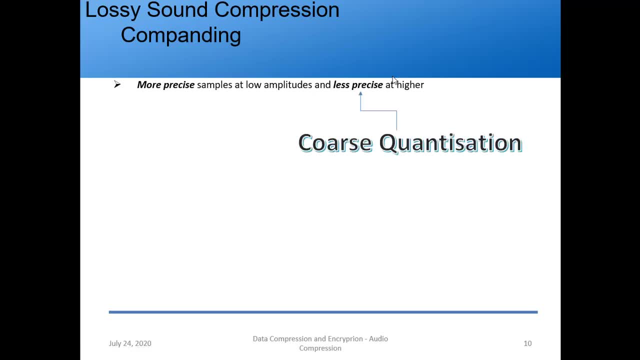 So quantization is changing right. So here it is fine, Here it is coarse. That is why compending is non-linear. So how we achieve compression using compending, For example, For 16-bit samples, we can encode using this formula, and this formula will give a output of 15 bits, right. 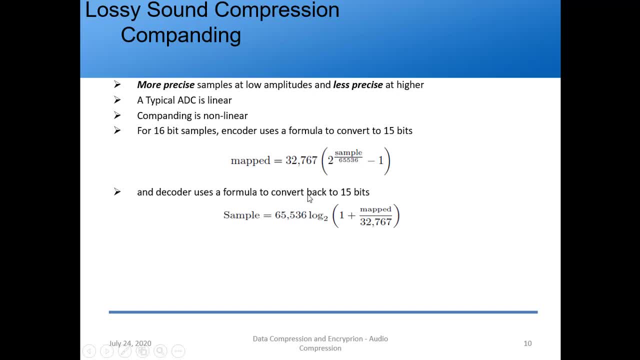 So, again, getting the original 16 bits. we use a decoder, So if we use that mapped expression here and use this formula, we will get the sample, original sample, which will be of 16 bits. So we are decompressing it. 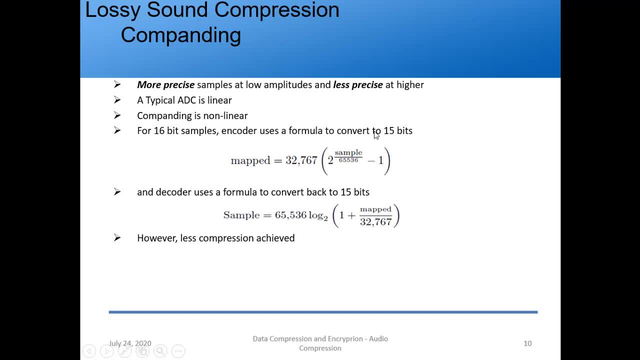 But what is the problem? We are only compressing 16 bits to 15 bits, So only 1 bit is getting reduced, So less compression is achieved. So what we do? So, instead of using this high number- 32, 7, 6, 7- we replace it by 127. 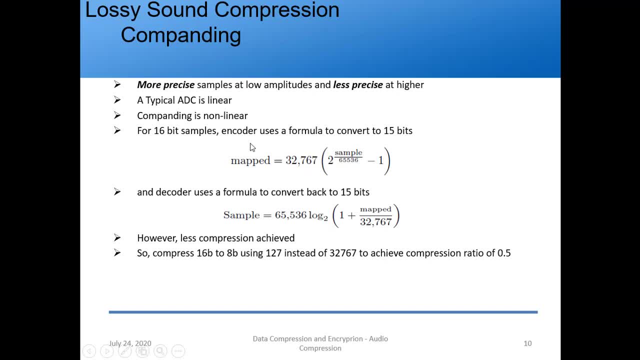 So if you replace this by 127, what happens? 16-bit number, instead of getting reduced to 15 bits, now gets reduced to what? 8 bits, right? So compression ratio achieved is how much 0.5.. So then we took the example of 60,100 and we saw that if we use 60,100 to convert from 16 bits to 15 bits, we get around 29,105, right? 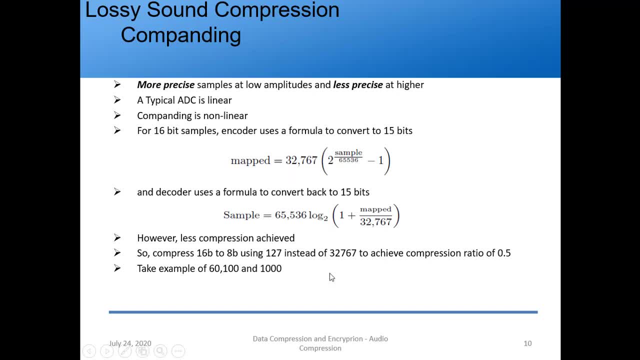 So 16 bits were converted to 15 bits. Then we instead of 32,, 7,, 6, 7, we used 127.. So we got the number was around 180, I suppose. So we got almost 0.5 compression ratio right. 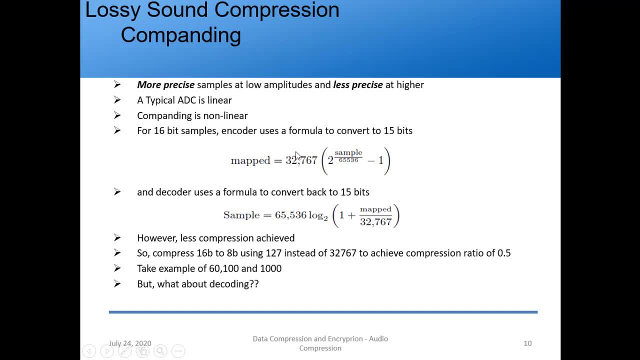 So what was the problem in decoding if you use 32,, 7,, 6,, 7?? It was highly iterative, right, Because errors were introduced low. But what was the advantage when you replace it by 127?? We knew the compression ratio in advance. 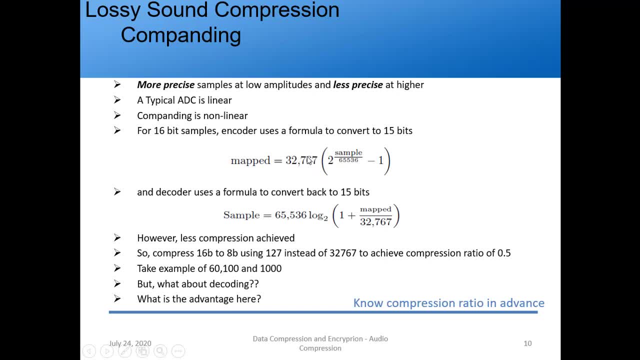 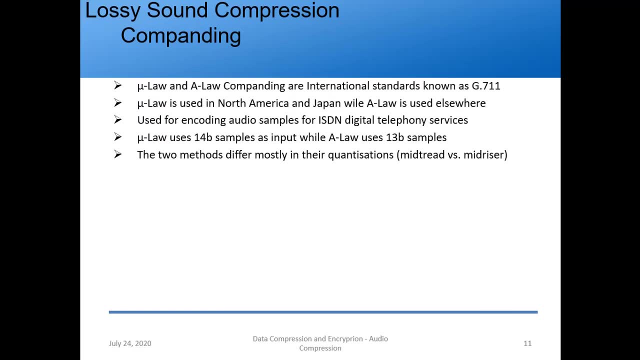 Right. So depending on the compression ratio we said we can change this value of 32,, 7,, 6,, 7 to our convenience. So accordingly we can achieve the compression ratio. So next we studied there are two compending type, 2 compending types. 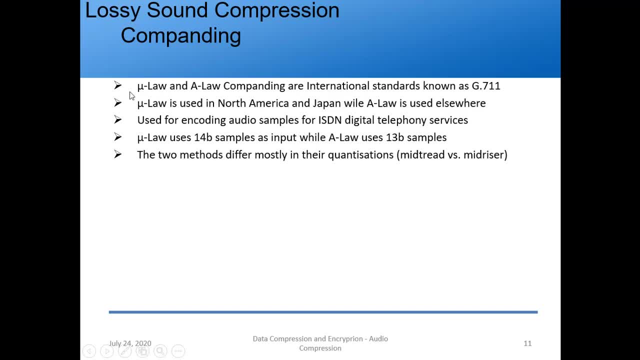 What are those MULA compending and ALA compending? So MULA and ALA compending are used in North America and Japan, while sorry, MULA is used in North America and Japan, while ALA is used elsewhere, right? 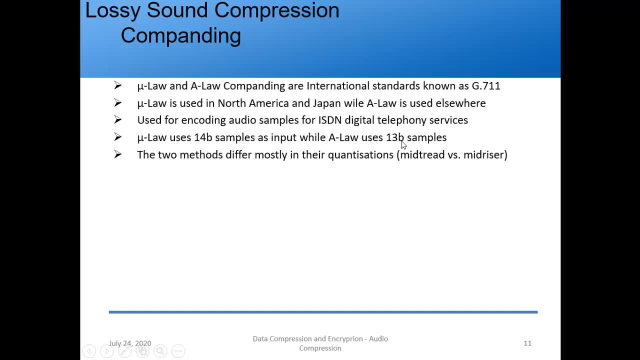 And MULA uses 14-bit sample. MULA uses 14-bit samples as input, while ALA uses 13-bit samples, And the two methods differ in the quantization, which is mid-trade and mid-trade. So these three differences are there. 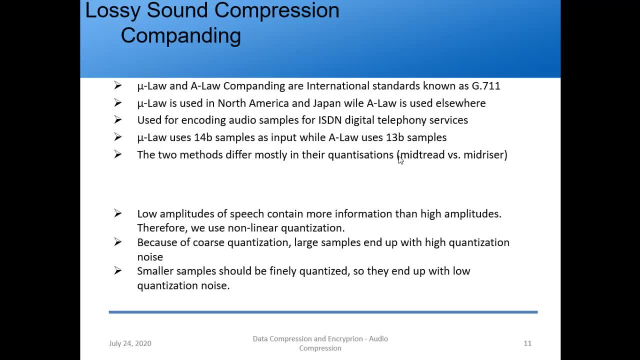 Then you can draw the diagram. So, as I said last lecture, these are important questions. Difference between MULA and ALA compending. So again, low amplitudes of speech contain more information. Therefore we use non-linear quantization. 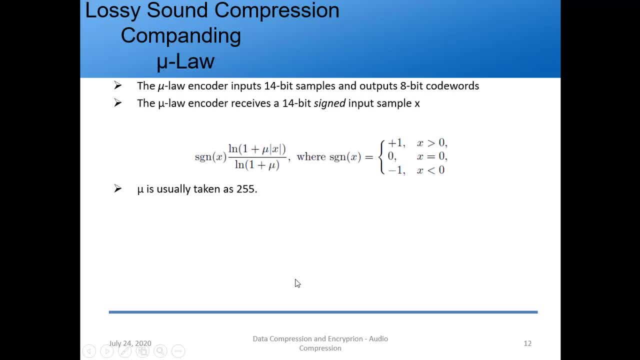 And smaller sample should be obviously finely quantized, right? So then, MULA: encoder inputs- what 14-bit samples? And outputs- 8-bit code words, right? So this was the formula. We will not discuss them. So this was very important. 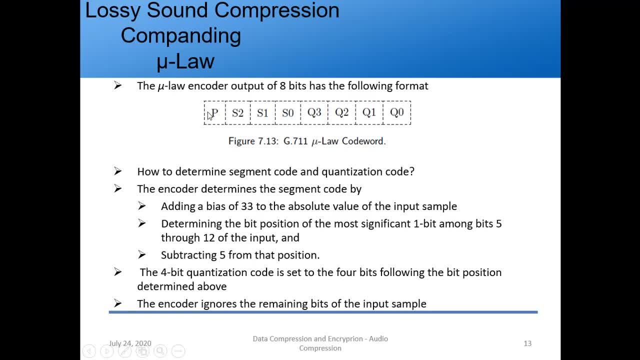 Again, the question comes on this: Usually they might give you a number And they will ask you to find the segment code and quantization code. So what you have to do, You have to use this formula. We have taken the example of minus 656.. 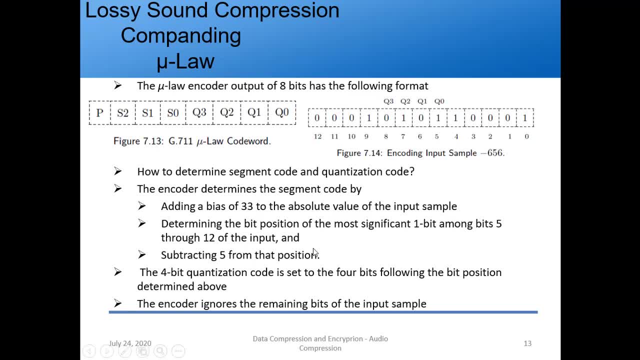 So, since it is minus, P will be 1. Then, using this procedure, we find the segment code And then, from that bit position which we get in the segment code process, We use it for quantization code, following that right. 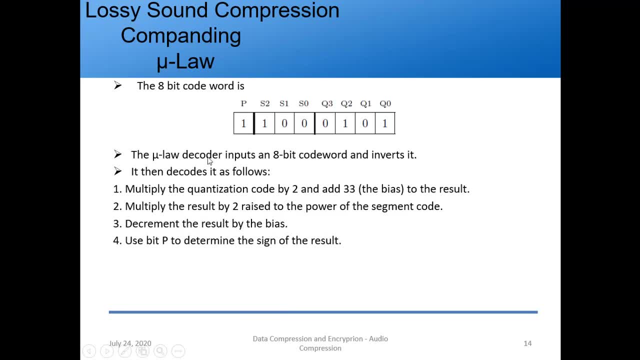 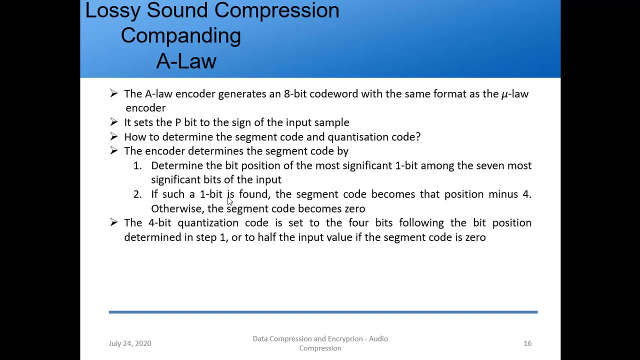 And the encoder ignores the remaining bits of the input sample right. So for decoding, again, we have the inverse formulas. So this is what we use for decoding right. So this is what we used yesterday, correct, And this was the diagram which we have to do. 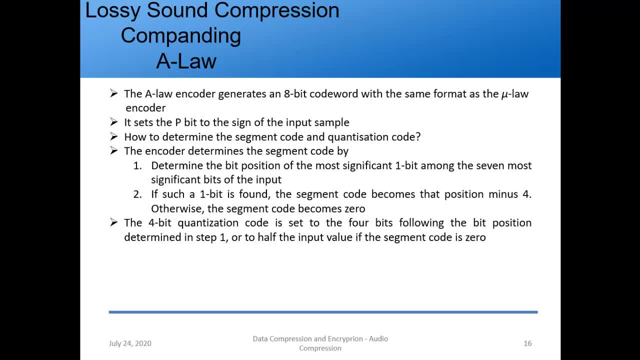 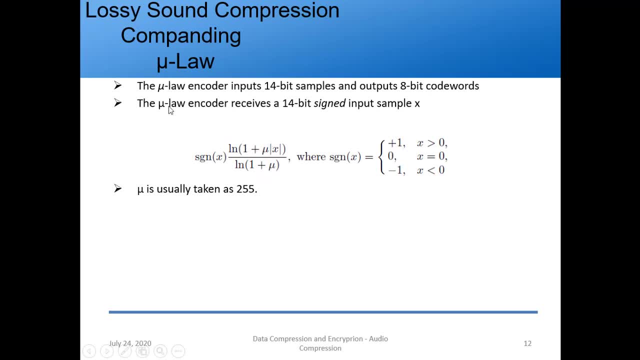 So let us proceed further. So next type of compending is Z-Law. What we have studied it was MULA. Why it is called as MULA? Because in the formula they have used mu. Because of this symbol, mu, it is called as MULA. 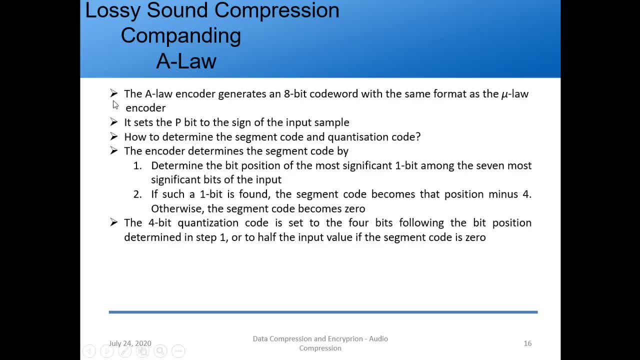 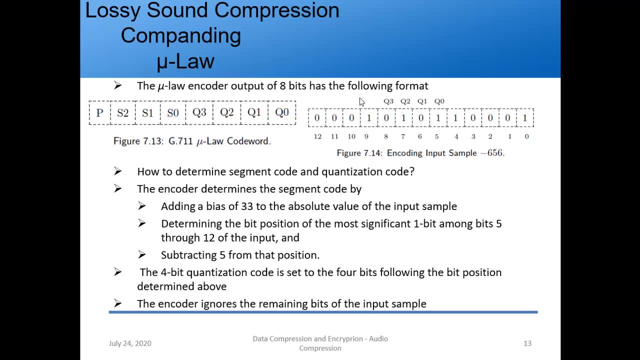 So then we have A-Law compending. So what does A-Law compending do? The A-Law encoder generates an 8-bit code word again. So yesterday I said we will see for the difference between MULA and A-Law compending question. 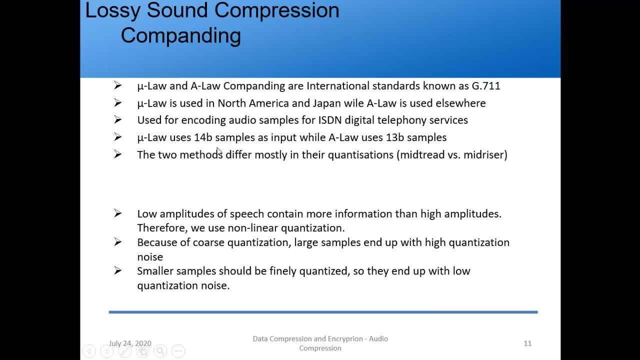 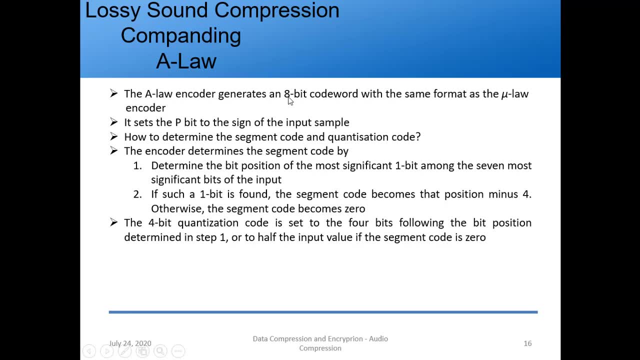 Let us see tomorrow what is the difference for output sample. So what is the output of MULA? It is 8 bits. What is it for A-Law? For A-Law also, it is 8 bits, right? So there is no difference with regards to the output. 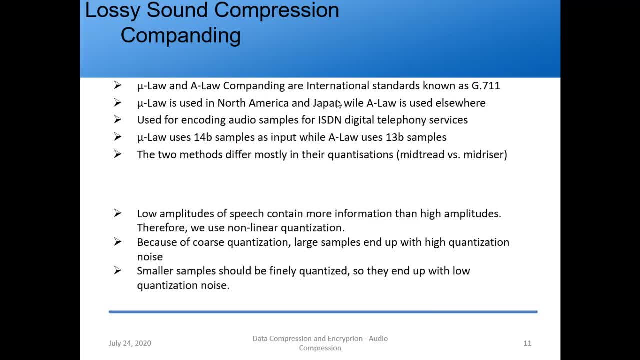 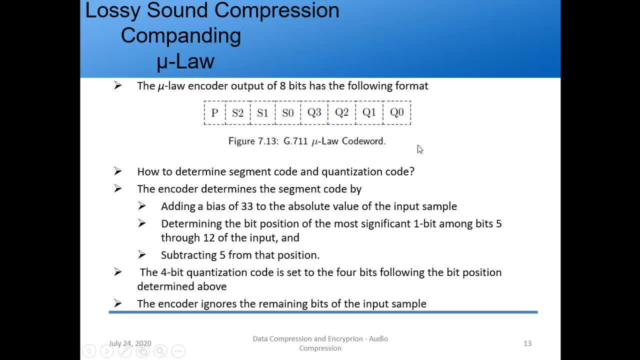 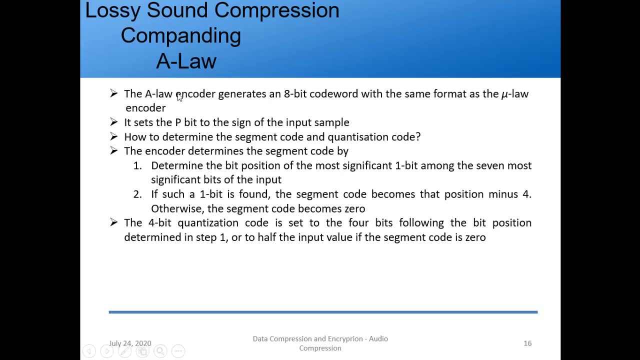 But with regards to input there is a difference, Because MULA uses 14-bit samples as input, while A-Law uses how much 13-bit samples. So again, the A-Law encoder generates an 8-bit code word with the same format as the MULA encoder. 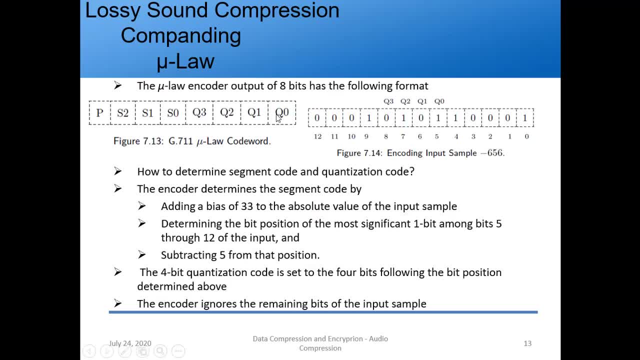 What does this mean? So this is the format for MULA, right? So this same format, that is, P, the parity bit, segment code S2, S1, S0- of 3 bits, Q3, Q2, Q1, Q0, quantization code of 4 bits. 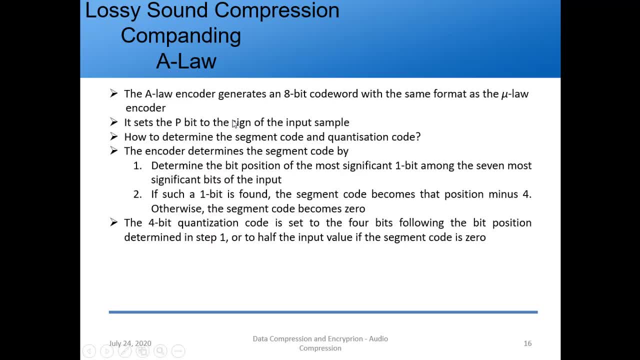 This same format is used by A-Law. So what does the B-bit do? P-bit do? It again sets the sign of the input sample. So then, what we do? Obviously, we determine the segment code and quantization code. 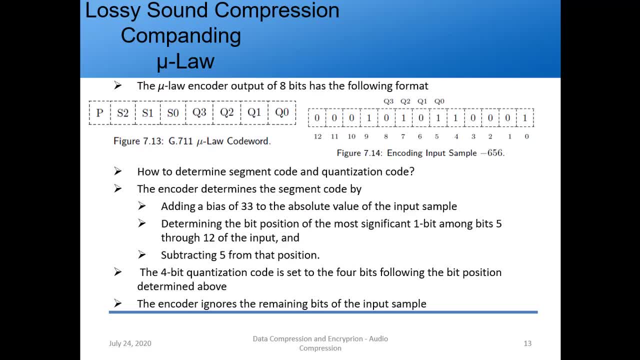 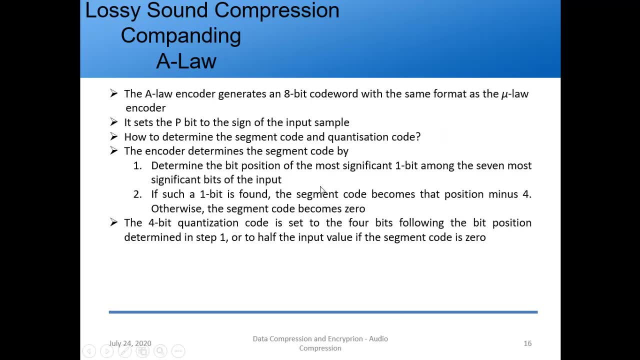 So if you see this procedure, this is similar to the procedure which we described For MULA, So I will not take an example, So I will just tell you the procedure. But in the exam they might give you a number and ask you to solve this. 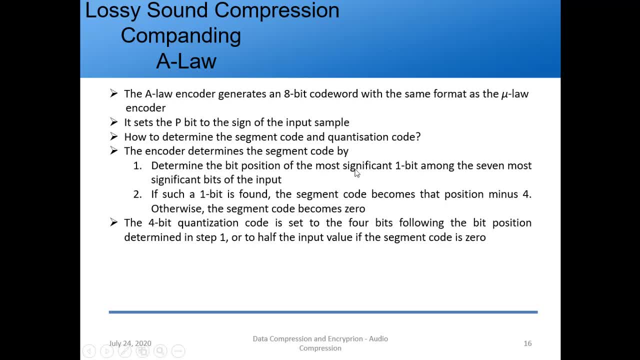 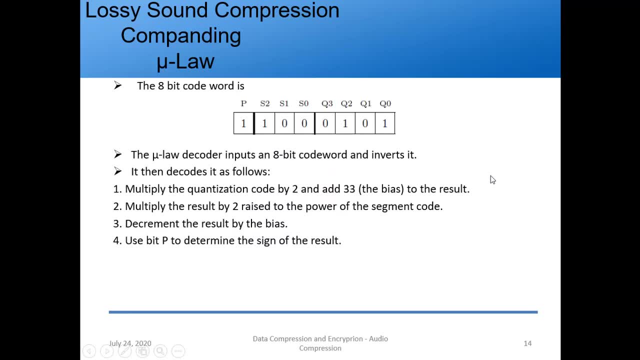 So the encoder determines the segment code by Determine the bit position of the most significant 1-bit among the 7 most significant bits of the input. Remember it is what 7 here Yesterday we saw it was different. Yesterday it was. 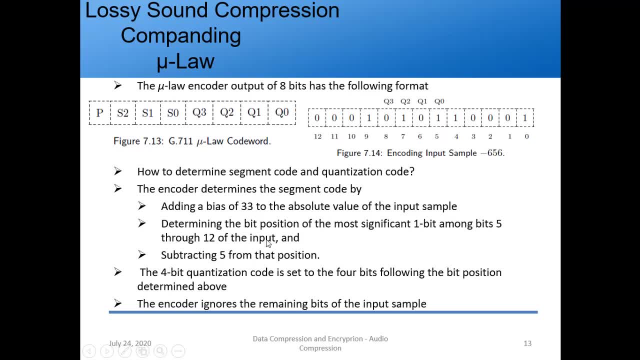 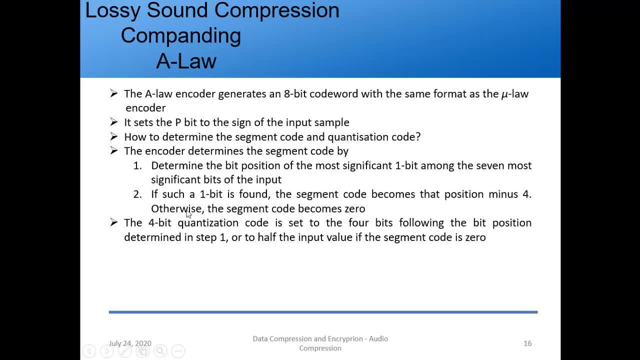 Bit position was most significant bit among bits 5 through 12. only Now it is among the 7 most significant bits. There it was 12 to 5.. So if such a 1-bit is found, the segment code becomes that position minus 4.. 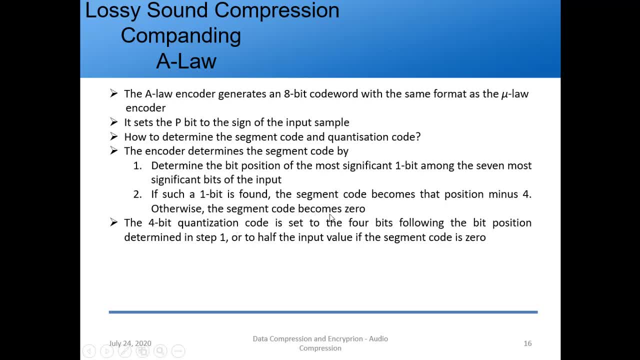 Otherwise, if this condition is not satisfied, the segment code becomes 0. Then we have to find the quantization code. So we find that the 4-bit quantization code is set to the 4 bits following the bit position determined in step 1.. 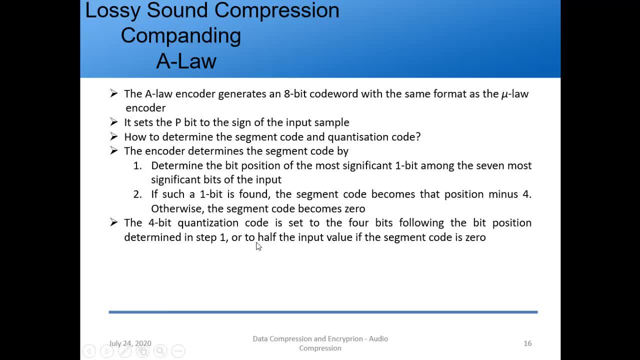 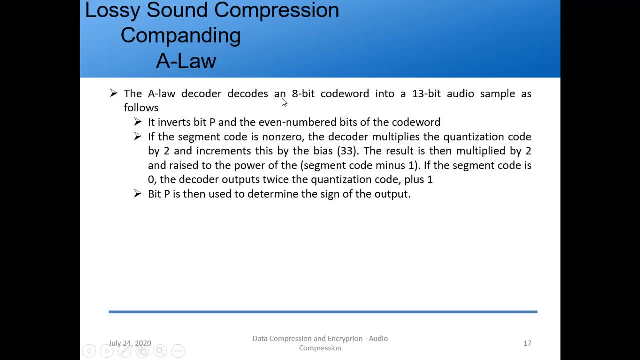 Or to half of the input value if the segment code is 0. So this is the same as the previous thing. Then about decoding. So again, 8-bit codeword, which was the output of encoder, will be used as the input. 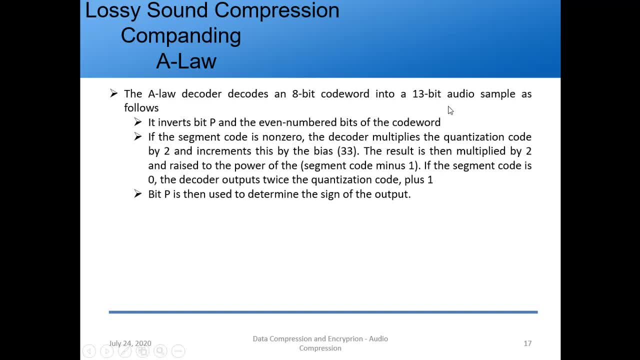 That is obvious. So we should get a 13-bit audio sample as output. So how we get that? So we use this procedure: First, invert the bit P and the even-numbered bits of the codeword. Then what we have to do. 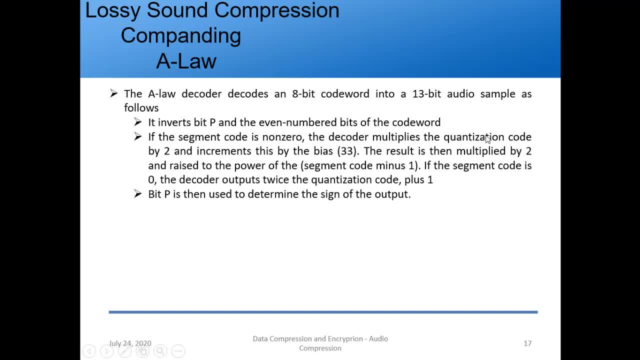 If the segment code is non-zero, the decoder multiplies the quantization code by 2 and increments this by the bias 33.. So same thing, Same as the MULO encoder. So the result is then multiplied by 2 and raised to the power of the segment code minus 1.. 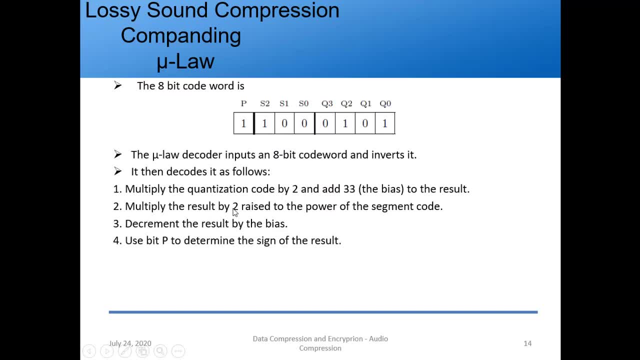 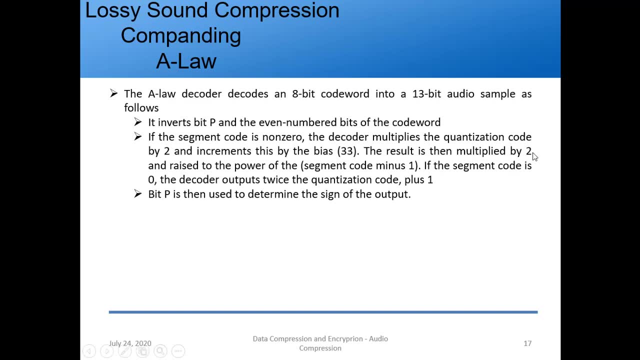 This is different. remember What we did for MULO decoder: Multiply the result by 2, raised to the power of segment code. Here, what we are doing: Multiply by 2 first and raise it to the power of the segment code minus 1.. 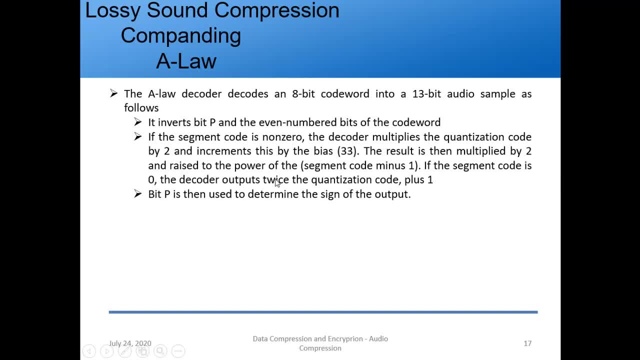 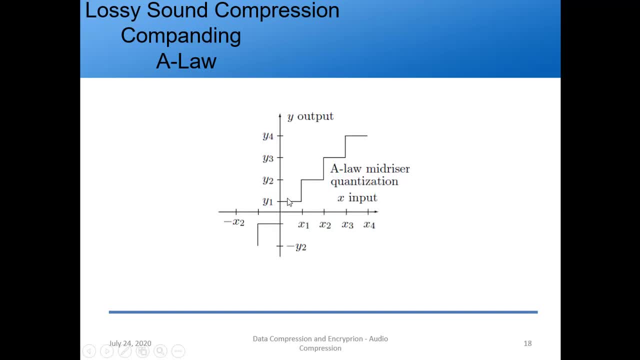 And if the segment code is 0,, the decoder outputs twice the quantization code plus 1.. So that's simple if segment code is 0. And bit P is then used to determine the sign of the output. Then we saw: 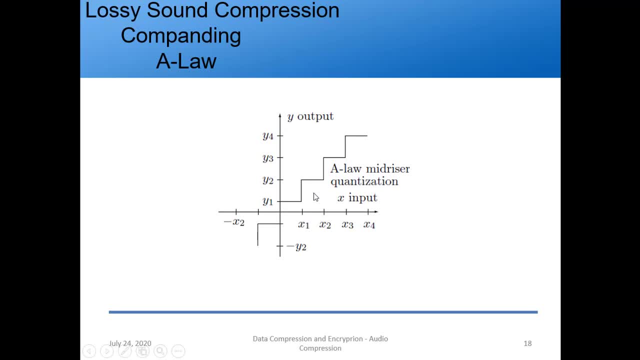 So this is the mid-riser quantization graph. So what is the difference between this MULO and ALOG in the graph? Here it is symmetric about the x-axis, Here it is along the y-axis. So that is the difference. 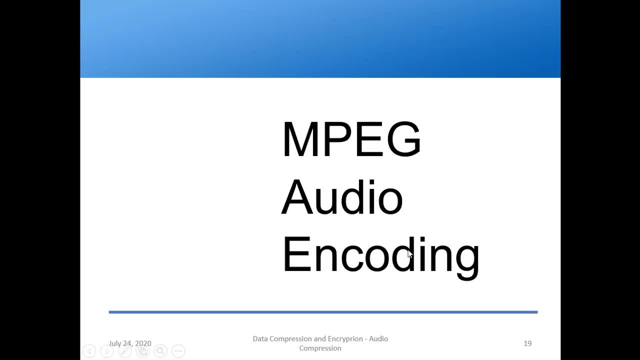 So then we have MPEG audio encoding. This is the next topic. So we are done with compending. So then we have MPEG audio encoding. So what is this? So this is nothing but our MP3 format. So this is the encoder and decoder block diagram. 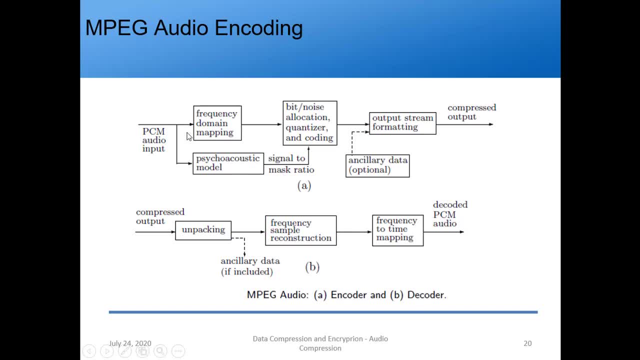 So just concentrate over this. You don't have to buy out this block diagram. You can just remember the blocks, But don't buy out what has to be written for each and every one. So for that, you just concentrate here. 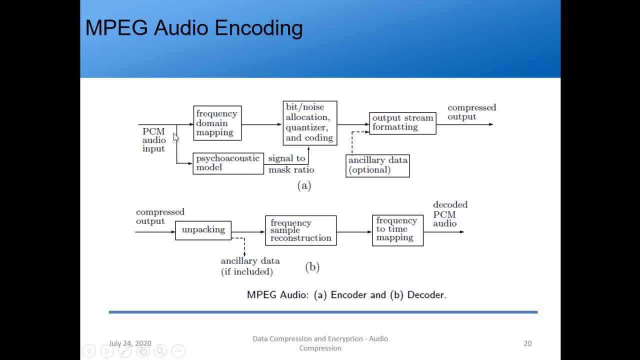 So what we have as input? Obviously we should have an audio input. So the audio input is our pulse code modulated input. So then it is given to the frequency domain. So the first question you should have is why we use frequency domain. 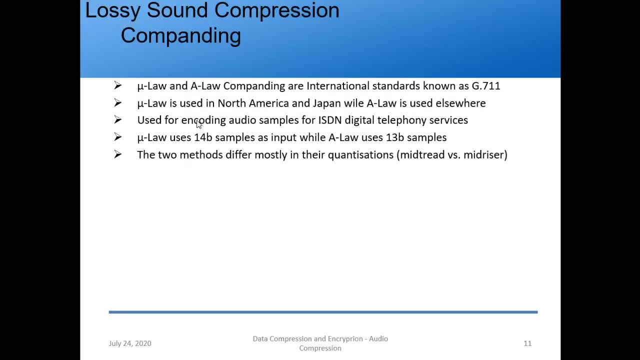 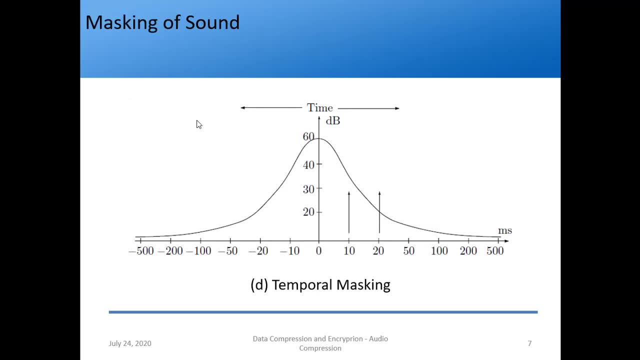 So for that, let's go to the very first or second slide which we used. Yeah, this was the slide, right? So hearing threshold: It is given in what terms? It is given in frequency. So x axis is frequency. 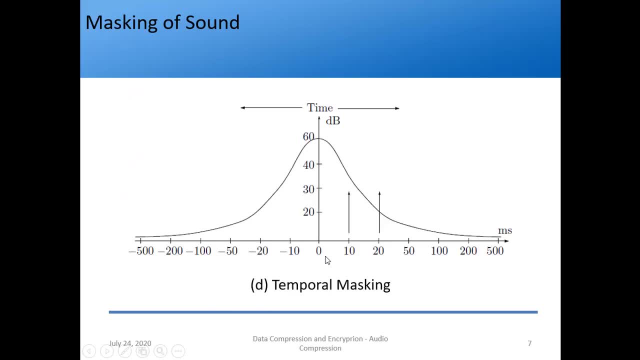 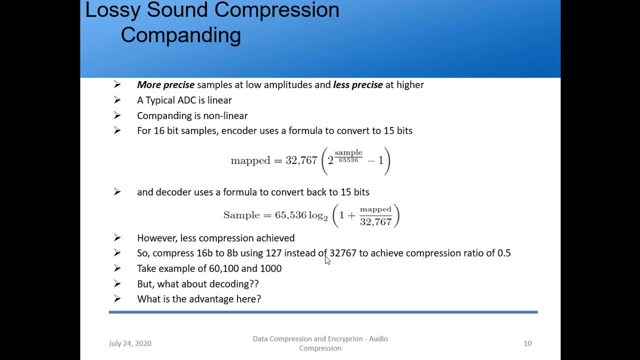 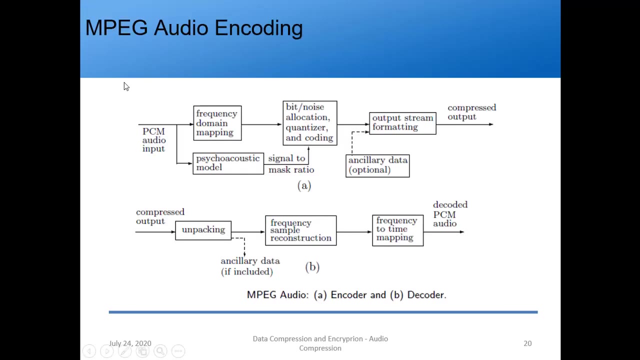 So sound is usually measured in frequency, right? So that is the reason we have the first block as frequency. So let's go to that slide. So have you understood why we are having first frequency? This is in what audio samples. 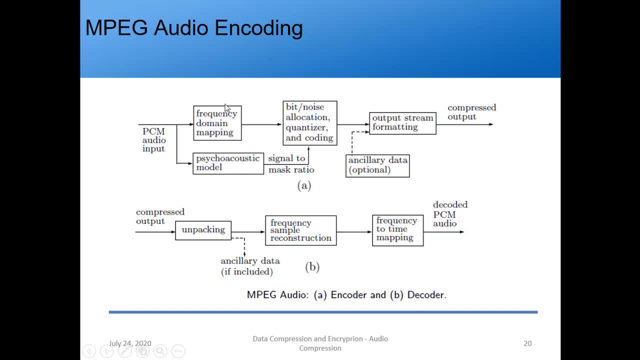 So we are converting those audio samples to frequency domain, right? So what you have to write here, I have just noted down in simple forms. So the frequency domain mapping is done in the sort of filters, form of filters And what those filters do. 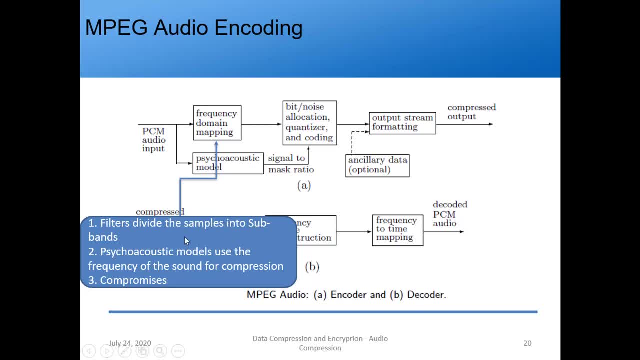 The filters divide the audio samples into 32 equal sub-bands. So what they do? again, They divide the audio samples into 32 equal sub-bands. okay, So what are these sub-bands and how they are converted Calculated? that we will see in the next further slides. 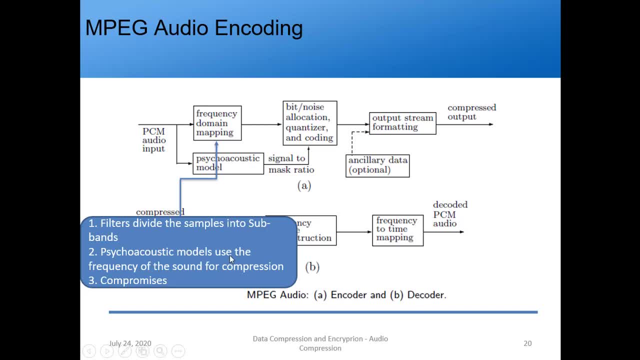 So then, psychoacoustic models are used, And through these psychoacoustic models the frequency of the sound for compression is determined. okay, So what is that? So that we will see here? okay, But what happens when we divide the samples into sub-bands? 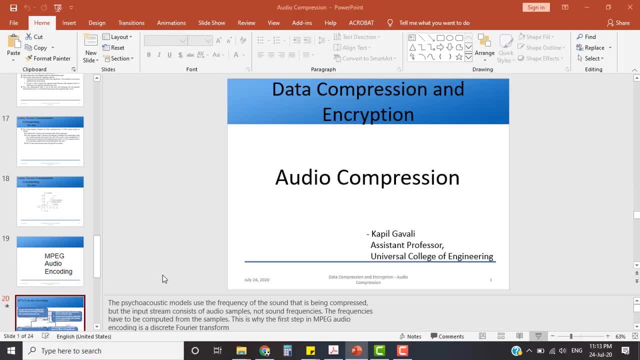 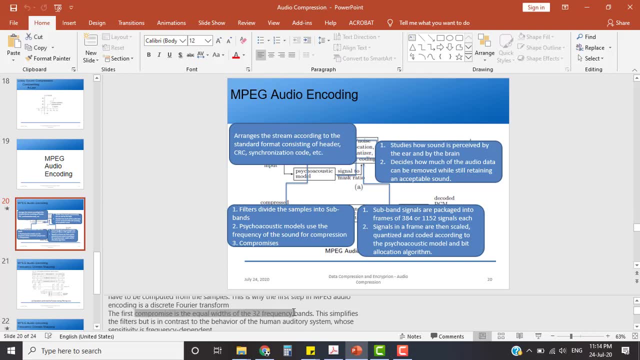 We are doing some compromises, So for that I have noted down in notes here. So what are the compromises? The first compromise is that the equal widths of sound Of 32 frequency sub-bands. So, as I said, these sub-bands are there. 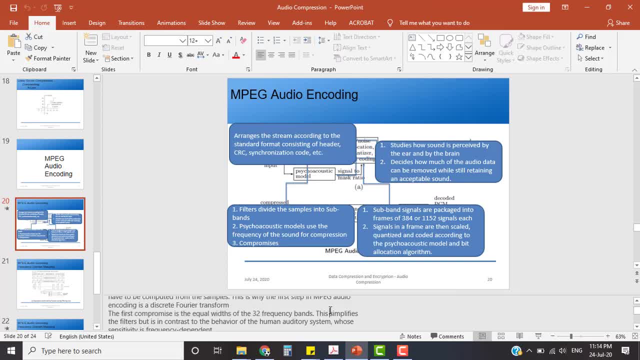 They are of equal widths. So what problem this does? This simplifies the filters, But what problem it does? This simplifies the filters but is in contrast to the behavior of the human auditory system, whose sensitivity is frequency dependent, right? So, since they are 32 equal frequency sub-bands, 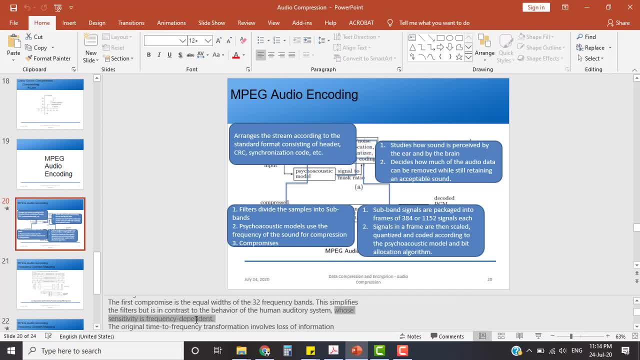 But our auditory system is designed to be frequency dependent, right? So it will create a problem, right? So then the original time to frequency transformation obviously will include loss of information, So some information is lost there. So that is the second compromise. 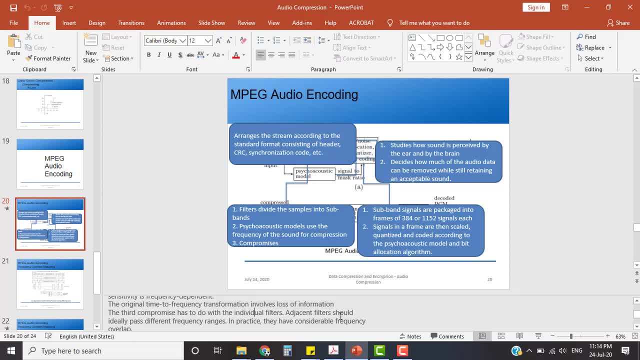 What is the third compromise? It has to do with the individual filters. Adjacent filters should ideally pass different frequency ranges, But as we saw there having equal sub-bands, So in practice they have considerable frequency overlap. okay, So these are the problems. 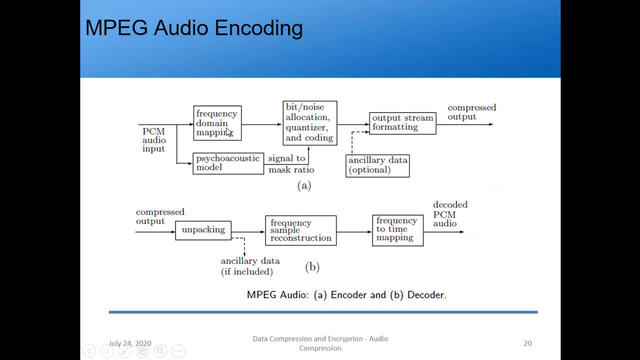 So you can just refer them from here, okay, So this is about what? Frequency domain mapping? So again, why we require frequency domain mapping: Because these are audio samples, right, So they need to be converted into frequency domain because we saw in the hearing threshold set it is usually in the form of frequency. 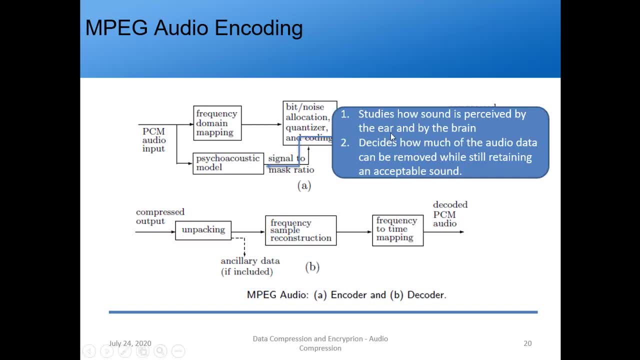 So next, psychoacoustic model. So what it does? It studies how sound is perceived by the ear and by the brain right And decides how much of the audio data can be removed While still retaining an acceptable sound. So this is basically. it just uses frequency. 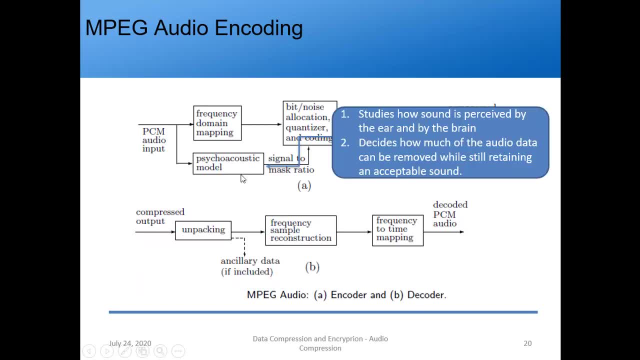 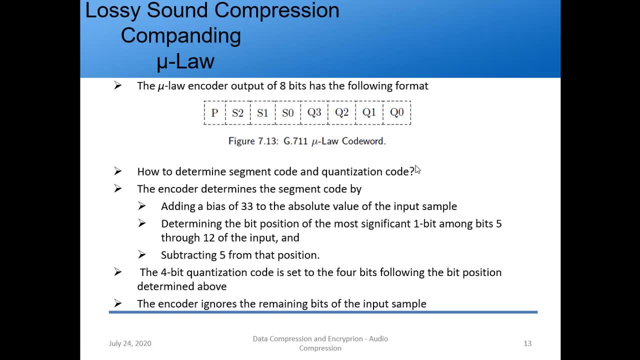 It just has the algorithms for frequency and temporal masking. So here it is what is written: Decides how much of the audio data can be removed. So how will it decide? So again, we can go to that masking slide. 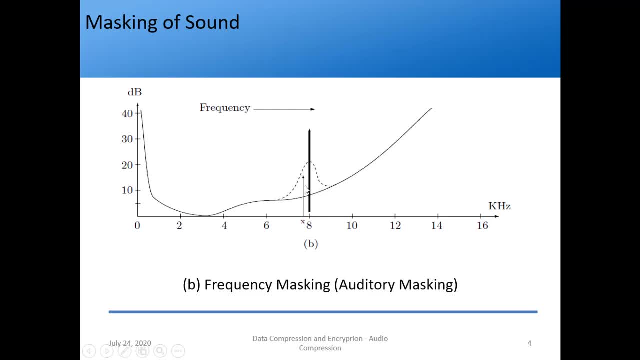 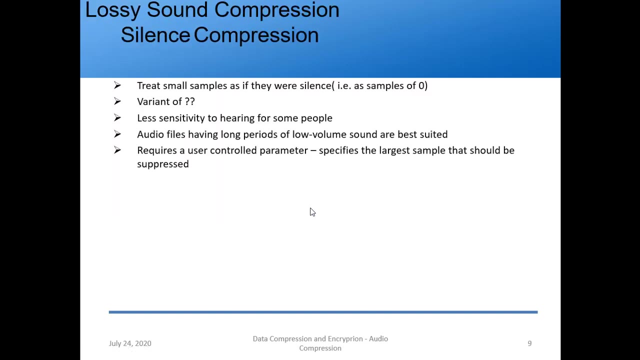 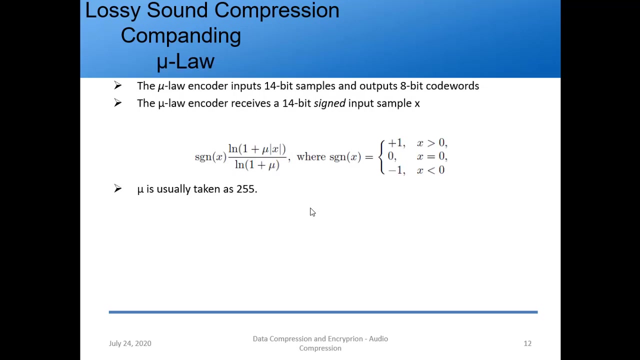 So from this diagram we saw that frequency at 8 kHz should be removed, right? So the psychoacoustic model is the one which decides which frequency component should be removed. So, based on this data, it will decide That frequency at 8 kHz should be removed. 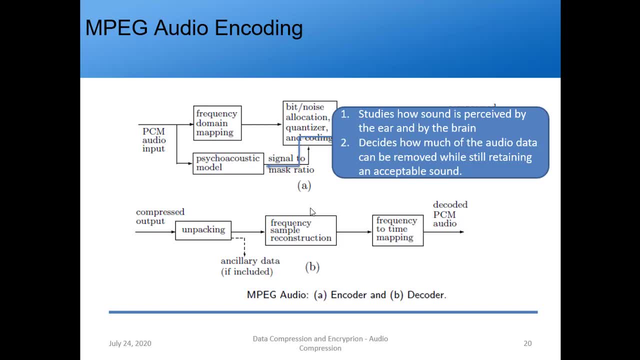 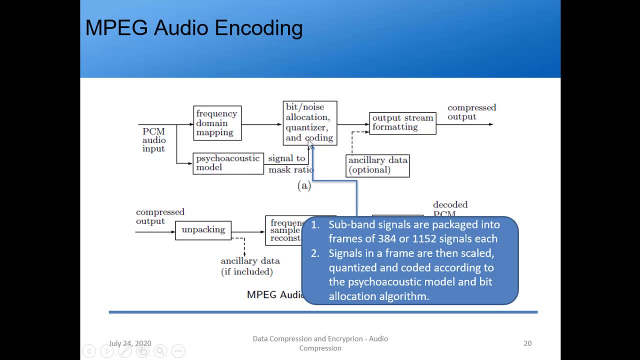 Let us go to the slide which we are using. Yeah, So this is what is done. by what Psychoacoustic model? Next, what we have. So this is the general step: Beat or noise allocation, quantizer and coding. 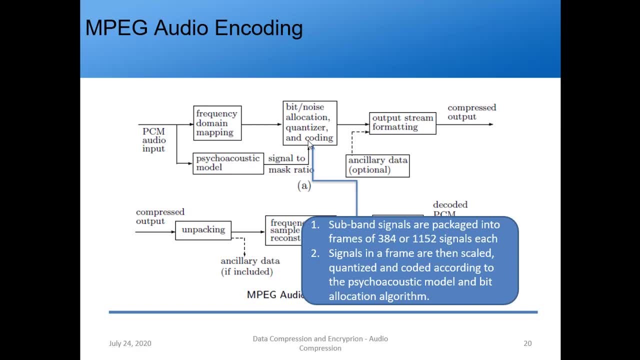 So in all the text and image compression and video compression models, So in all the text and image compression and video compression models we saw, the penultimate or the ultimate step is what We saw. the penultimate or the ultimate step is what 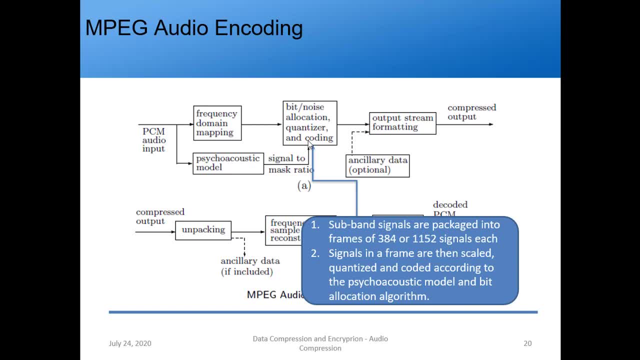 Encoding. Encoding, So either they use QM coder or Huffman coding or arithmetic coding right, So either they use QM coder or Huffman coding or arithmetic coding right, So either they use QM coder or Huffman coding or arithmetic coding right. 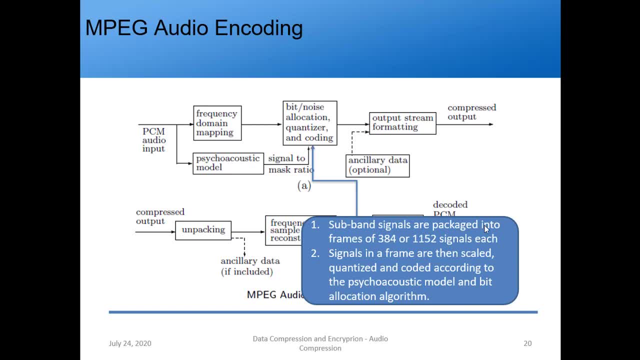 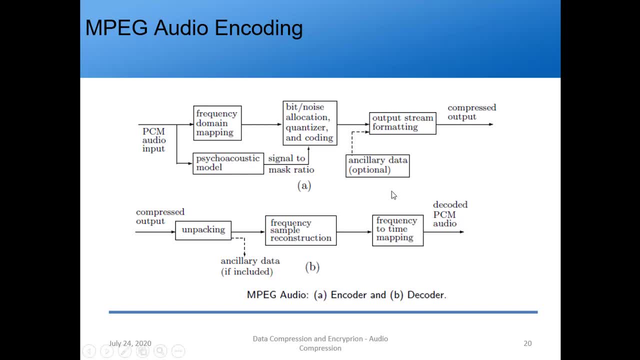 So subband signals are first packaged into frames of 384 or 1152 signals each out. so this is about what encoder, right? so what? we decode the recorder, so this output is given as input to the decoder, so it unpacks the data and then frequency sample reconstruction. so that is. 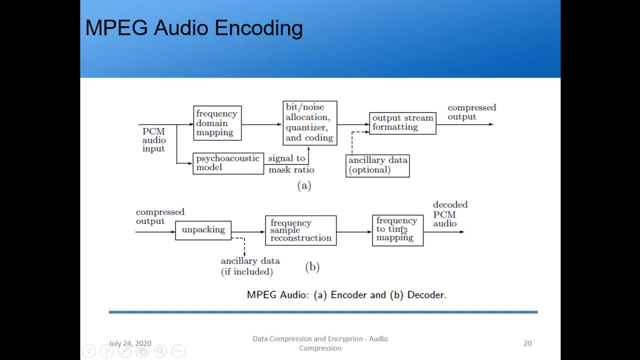 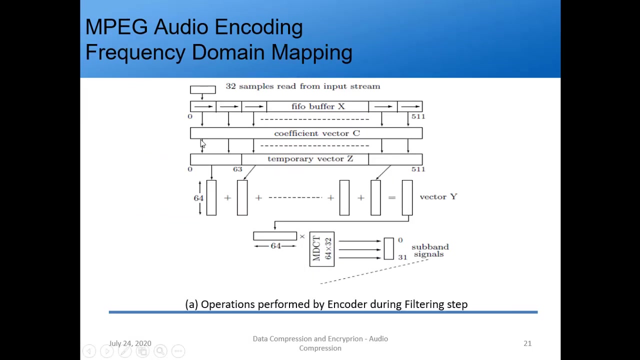 from this data it is again getting the frequency components then, since we have done frequency domain mapping, so from frequency domain mapping again we get the original decoded pcm model. okay, so then i said how this frequency domain mapping converts into 32 sub bands here. right, so let's see that. so this is the what is happening inside the frequency. 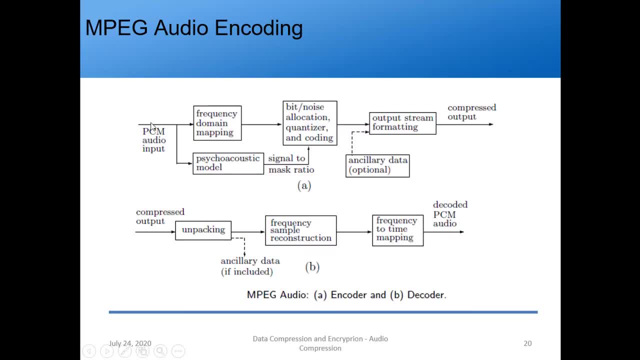 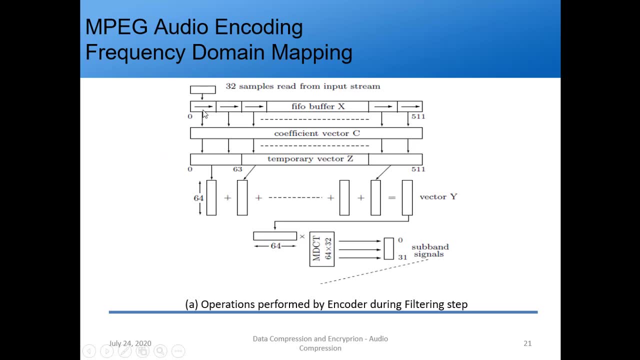 domain mapping. so what we have- we have audio samples here, right? so what the frequency domain mapping block does is it takes the first 32 samples, so it puts them in the first in first out buffer, which is named, as in the standard format, �uit format as x. so it takes those, then it shifts them to the rate when the next 32 samples 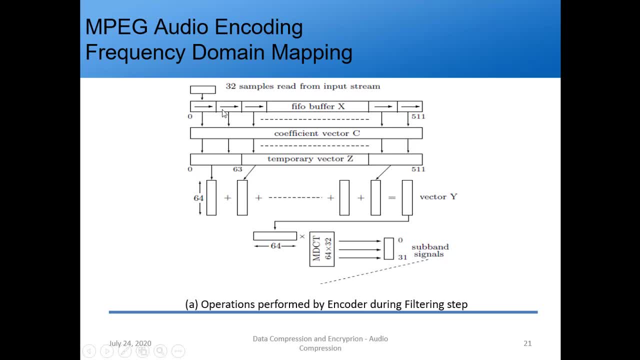 will come, it will shift them to the rate. then it will next 32 samples will come. so like this it can store up to total 512 samples. so once these 512 samples are complete, what it does? they have a coefficient vector c. so we saw in dct that there is a quantization table. it is given by the jpeg. 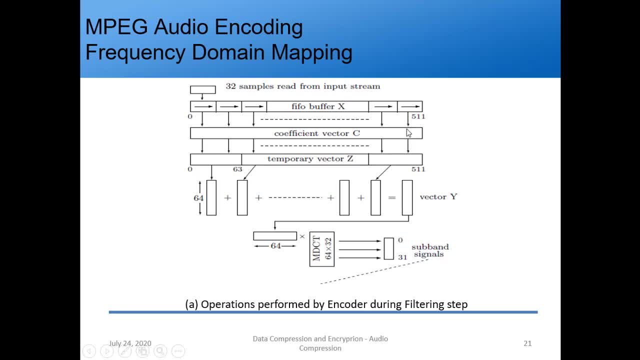 team right. so in the same way, this coefficient vector c consists of coefficient values which are given by the impacting, multiplies this each 32 bit numbers by this coefficient vector so that we get each 32 numbers here in the blocks here. but what it does for the temporary 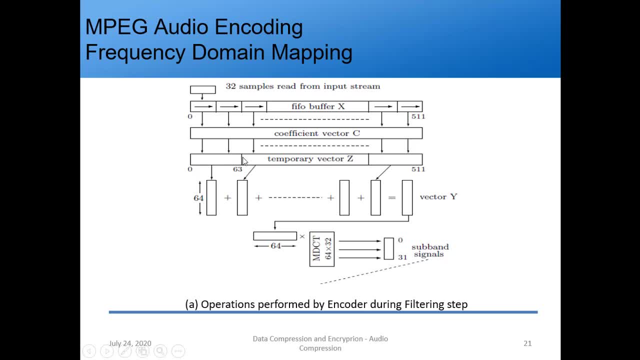 vector Z is it takes 2 times 32, that it is makes one block of 64 samples. so like this it will make total 0 to 512, right? so it will be how much? I think it will be 8, so this will be 8 matrices. I suppose you can just divide 512 by 64. 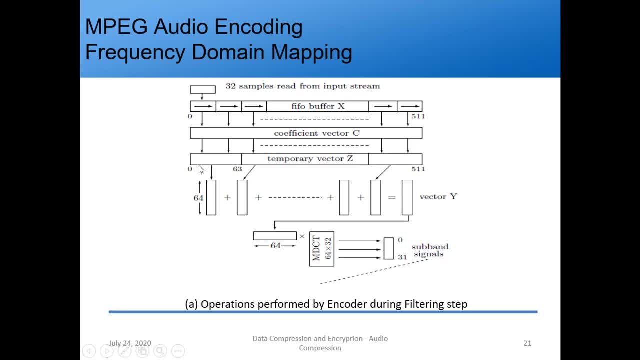 then we will get that. so next what we do. so these are rules, right. so the software or the algorithm will convert them to columns and then add them. so after adding them, we will get a vector Y. so this vector Y is almost size 64. so this 64 is again taken as a row and multiplied by a modified DCT transform. 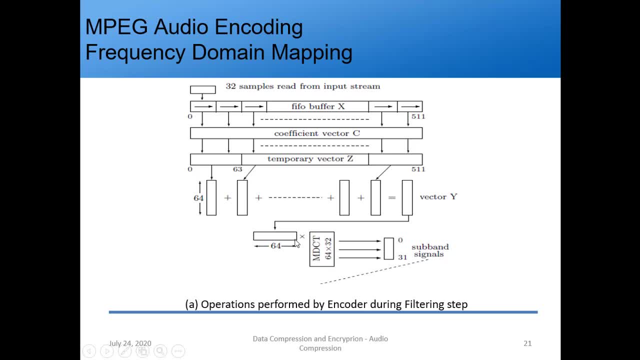 so, again, we are using DCT, right, so this is 1 by 64, this is 64 by 32, so we get a column vector of 32 sub band signals. so what we have done- 32 the audio samples we have converted to 32 equal sub bands- right? so this is what is done by the encoder. 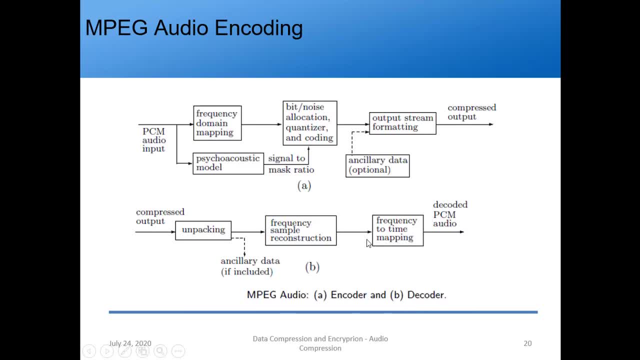 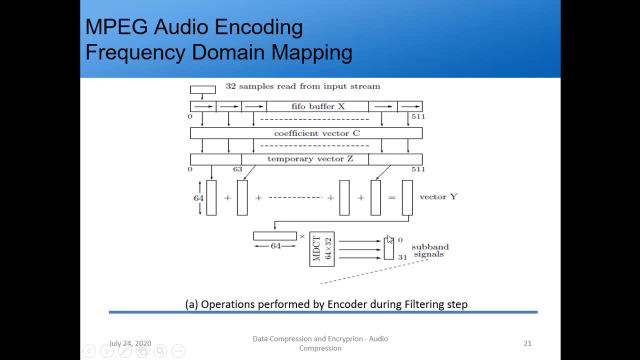 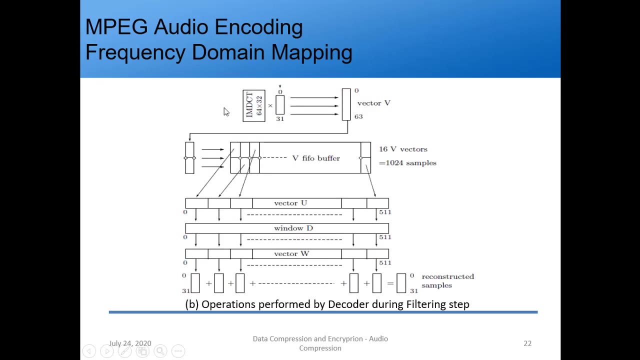 during filtering step. so what happens here? frequency is to time domain, so that we'll see in the decoder step. so we have that original 31 bit samples. so this sub band signals are nothing but taken here. so, and corresponding to the MDCT we have, I am DCT. that is the inverse transfer. so we multiply them, we. 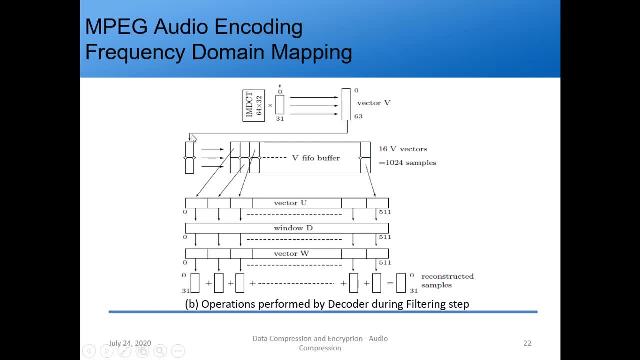 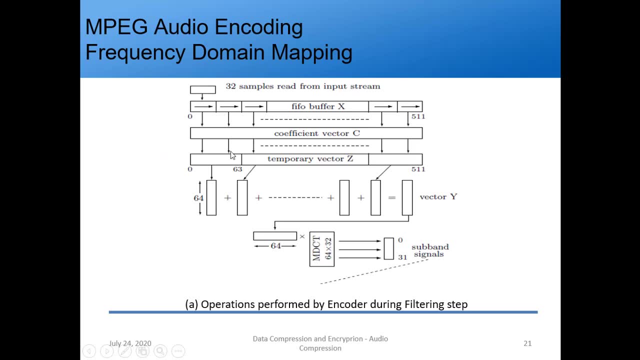 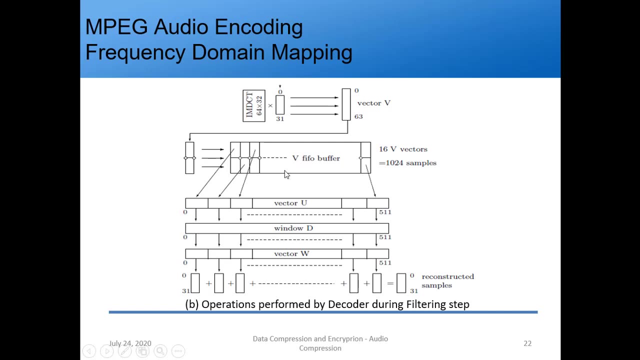 again get 64 vectors right. so in the same way that this 32 samples will be coming from, the audio rate will continue. the audio samples will be continuously coming. so in the same way, this 32 samples will continuously becoming so we will have that first 64 vector V. so we will fill them in the FIFO buffer. so 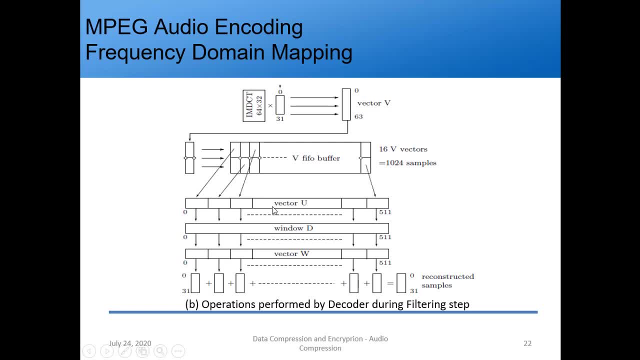 once one zero two four samples are completed, it will give them in the vector 2. so this vector 2 will be divided into 32 bits. again, 32 samples or one. so one zero two four samples are finished. so once this 51 to our field it.